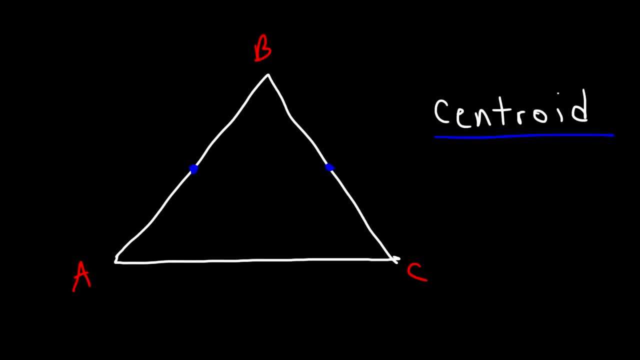 So let's identify the three medians of a triangle And then draw a line from the vertex to the midpoint of each side, And then draw a line from the vertex to the midpoint of the other side, So the centroid is approximately in that region. 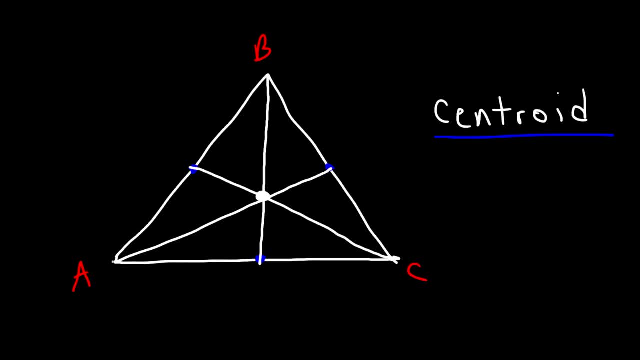 So, like the in-center, the centroid always lies inside of the triangle. So let's call this Point D, E and F And let's call this point P. Now it turns out that AP is two-thirds of AE And PE is one-third of AE. 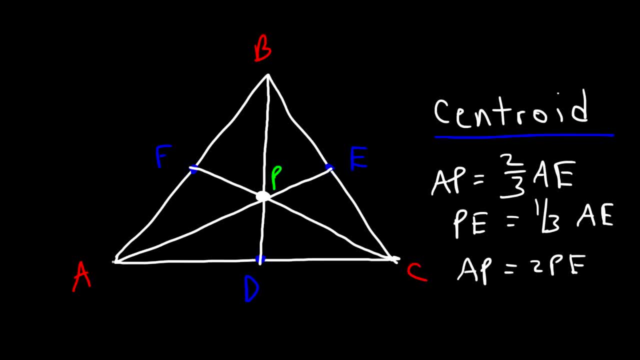 And AP is twice the value of PE. So let's say, if PE is 5,, AP is 10.. If FP is 4, PC is twice the value, it's 8.. If BP is 12, PD is half the value, it's 6.. 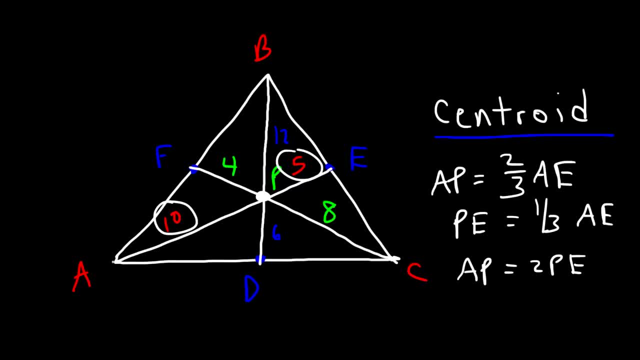 Now the total length of AE: 10 plus 5, that's 15.. We can see that AP is two-thirds of 15.. Two-thirds of 15 is 10.. PE is one-third of 15.. One-third of 15 is 5.. 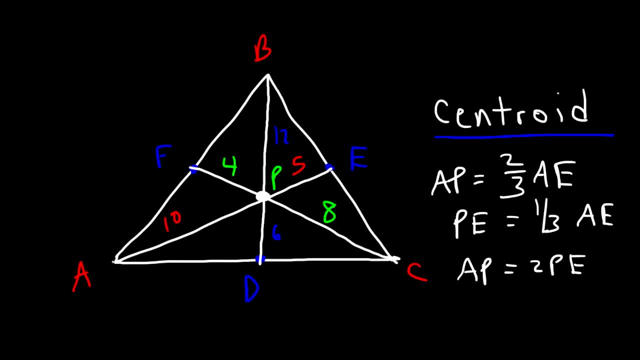 And so any time you have a centroid, the long side or the long segment will be twice the value of the short segment. So to review, the centroid inside a triangle can be identified by the intersection of the three medians. So if AE is the median, that means E is the midpoint of BC. 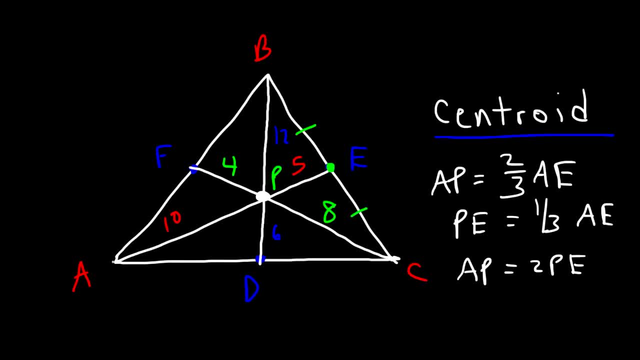 Which means that BE and EC are congruent. Now, BD is the median to AC, so D is the midpoint of AC, so AD and DC have to be congruent. F is the midpoint of AB, since FC is the median, So FB and AF are congruent. 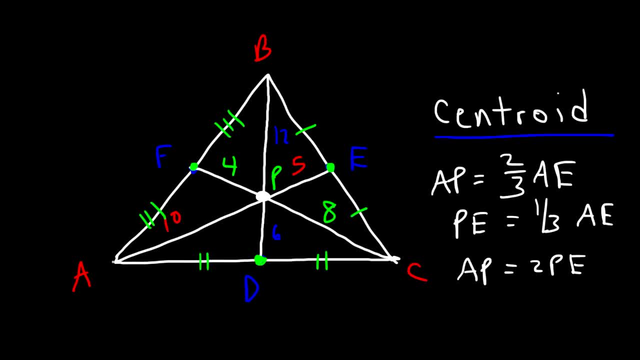 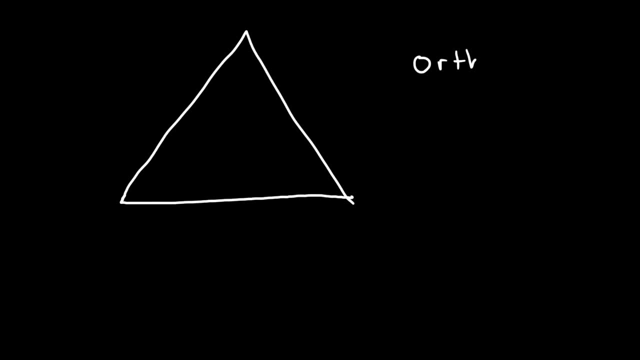 The orthocenter of a triangle. Now, the orthocenter doesn't have to lie inside of the triangle. It can be on a triangle or outside of the triangle. Now if we have an acute triangle, like this particular example, it's going to lie inside. 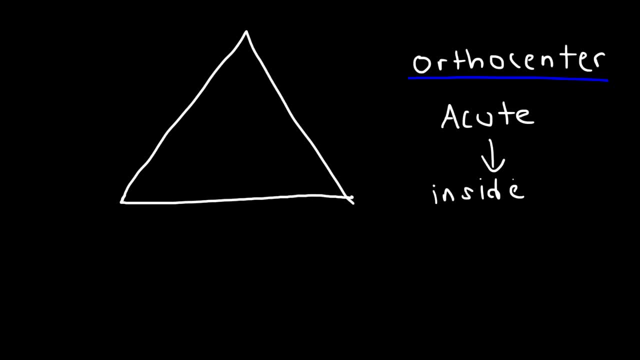 of the acute triangle. If we have a right triangle, it lies on the right triangle And if we have an obtuse triangle, it lies on the right triangle triangle. it's going to lie outside of the obtuse triangle. Now the location of 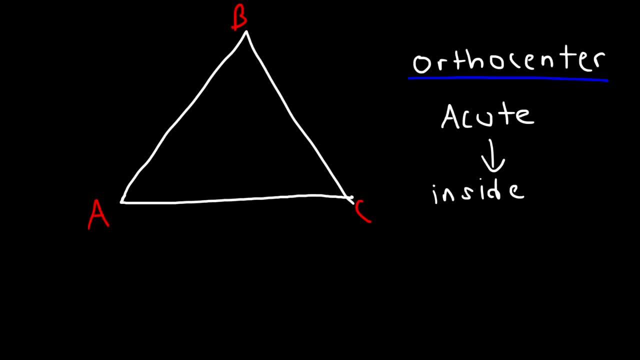 the orthocenter can be found by the intersection of the three altitudes. So let's draw an altitude from vertex A to the opposite side side BC. So we need to draw in such a way that it's perpendicular to the opposite side, which 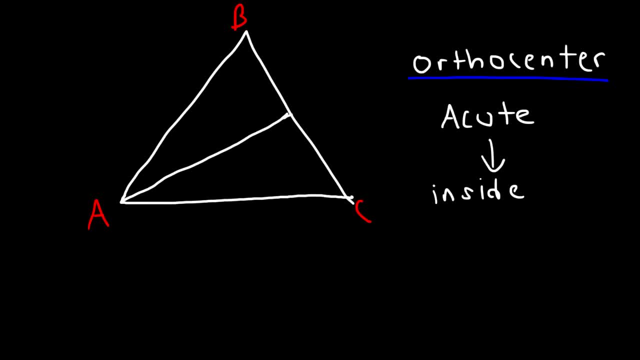 is probably going to be around here. It looks perpendicular at that point. And then do the same for vertex C. So around there should be perpendicular. And then let's draw a line from B to AC. So, as we can see, the orthocenter is approximately: 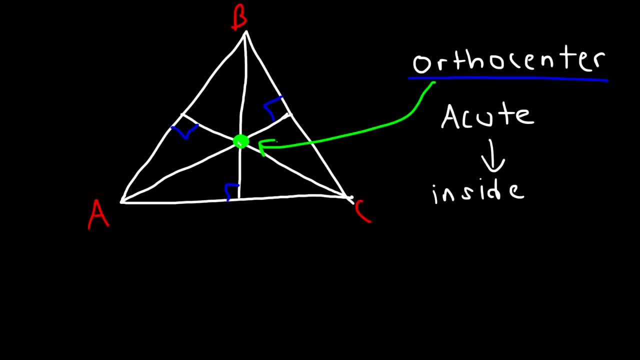 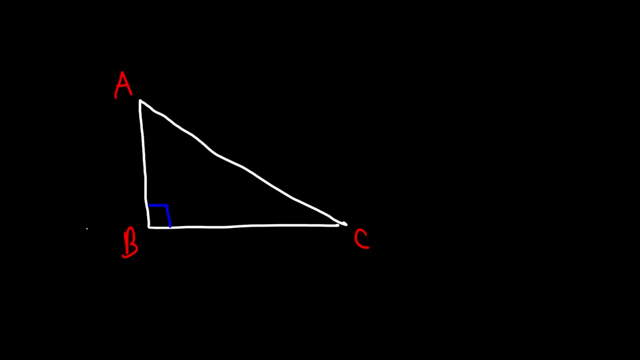 somewhere in this region. So if you have an acute triangle, the orthocenter lies inside of the acute triangle. Now let's focus on the right triangle, Let's identify the location of the orthocenter. So first let's extend each side. So I'm going to extend side BC, side AB and also 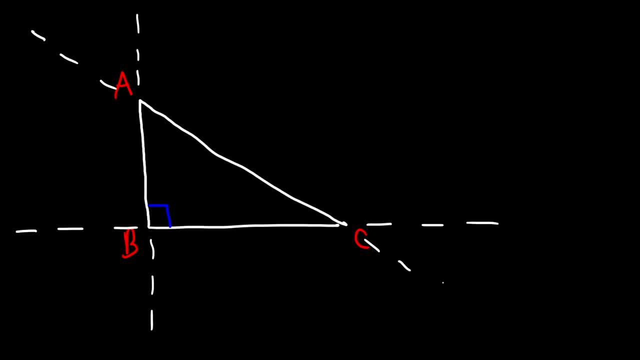 I probably don't need to do that, but I'm going to do it anyway. So what we need to do is draw an altitude from vertex A to B? C And notice that the altitude is here, because that's where it meets B? C at a right angle. 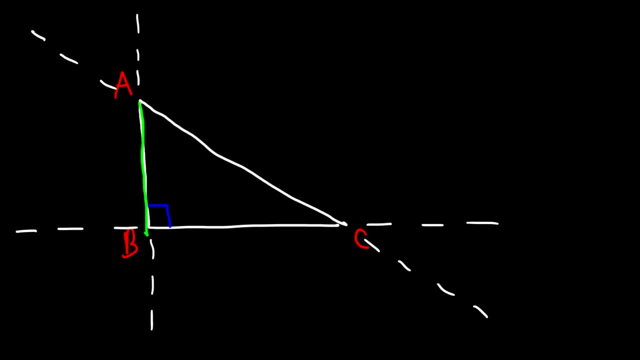 So this is the altitude from vertex A to B, C. Now let's draw the altitude from vertex C to side AB. So that's going to be here because it's perpendicular to side AB. Now let's draw the altitude from vertex B to AC. 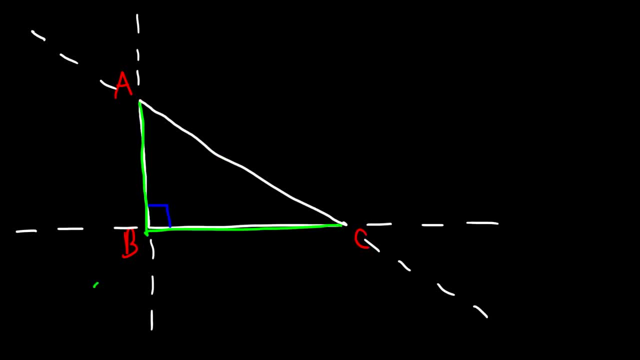 So that's going to be actually. let's do that again. it should be like this: Okay, this is approximately a right angle. It's not exactly 90. It's close to it. I have a case. you can see that this is the location of the orthocenter. 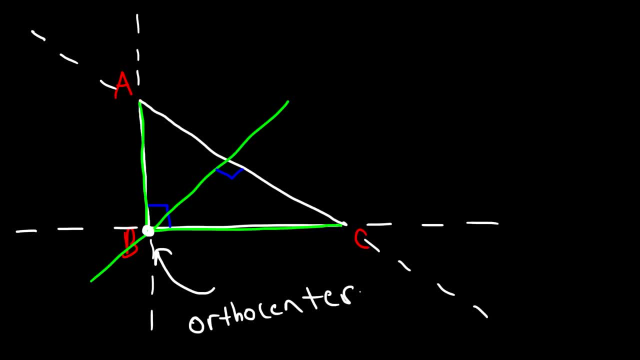 The orthocenter is located at the right angle of a right triangle. So let's say, if this is the right triangle, The orthocenter will be located at the right angle, Or if we have another right triangle that looks like this, the orthocenter is going. 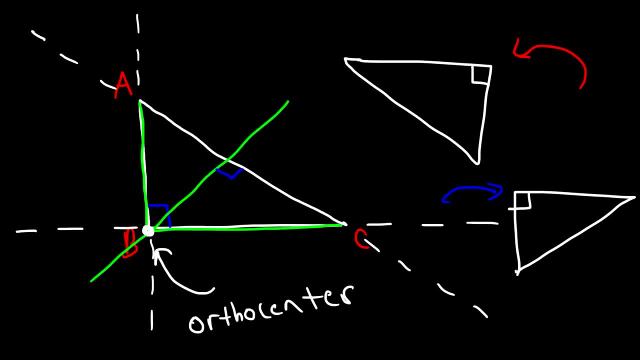 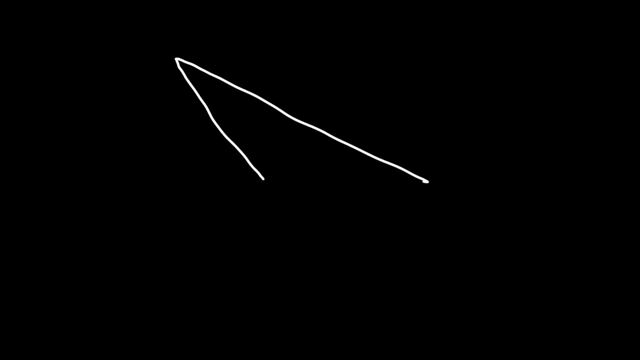 to be located right there, And so that's how you can identify the orthocenter of a right triangle. It's always located on the right triangle, at the right angle. Now, what if we have an obtuse triangle? So let's call this A, B and C. 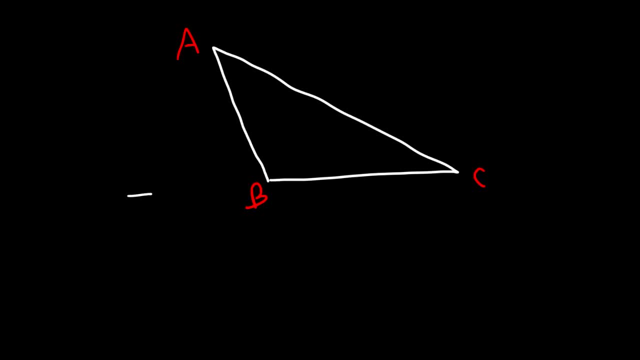 So I'm going to extend each side. So let's call this A, B and C. So I'm going to extend each side. So let's call this A, B and C. So I'm going to extend each side. 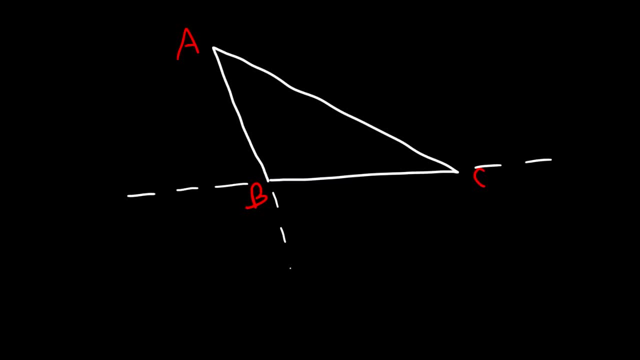 This is B, C And here we have A, B And let's extend A C. Let me do that again. So let's draw the altitude starting from vertex B to the opposite side, A, C, I'm going to. 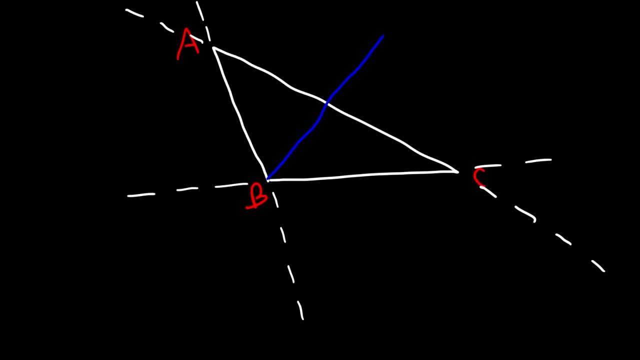 do it in blue. Okay, So this is the right angle. So this is the right angle. And then let's draw the altitude from vertex A to side B, C. So remember it has to be perpendicular. So notice that it's perpendicular at B, C at this point. 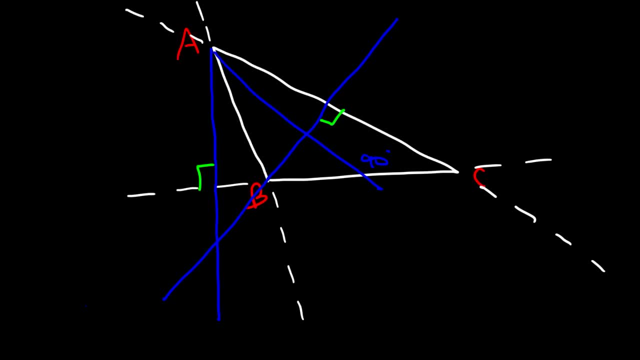 If you draw it here, this is not going to be a 90 degree angle, So let's draw it here. So, for an obtuse triangle, we can see that the orthocenter is going to lie outside of the obtuse triangle. 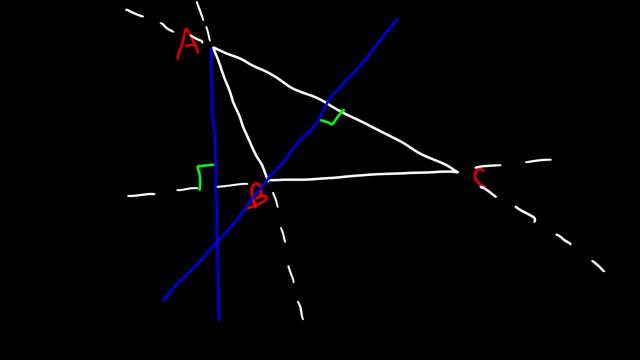 Now let's draw the third line, And it's going to be from vertex C, perpendicular to A, B, And so we can see here it's approximately 90 degrees, And so they intersect at that region. So that's the orthocenter of an obtuse triangle. 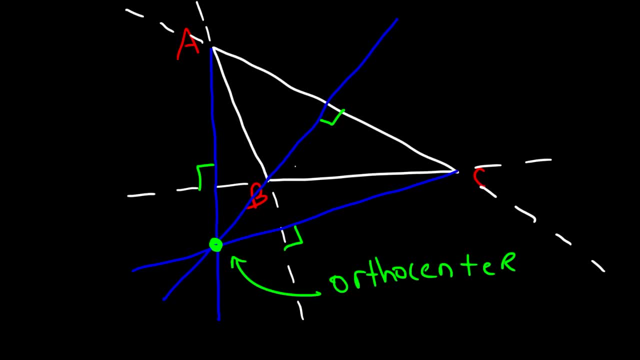 An obtuse triangle is a triangle that has one angle that's greater than 90. So this angle is more than 90. It could be like maybe 110. That makes it an obtuse triangle. So now you know how to identify an orthocenter. 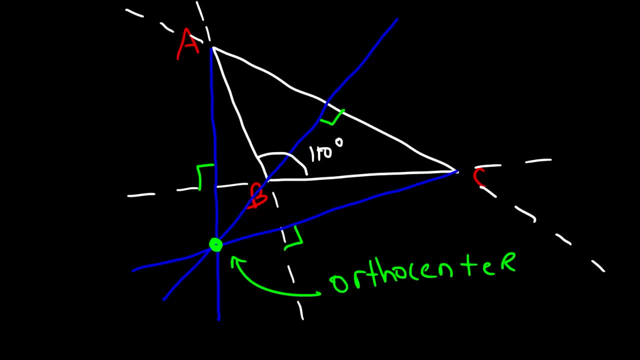 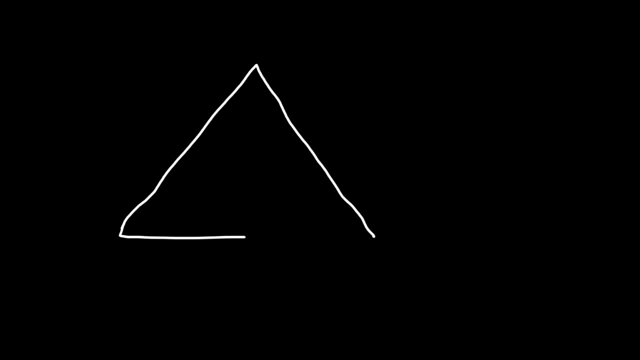 It's the location where all three altitudes of a triangle intersect. Now there's one more term that we need to go over, And that is the angle that is greater than 90.. Okay, And that is the circumcenter. So how can we identify the location of the circumcenter? 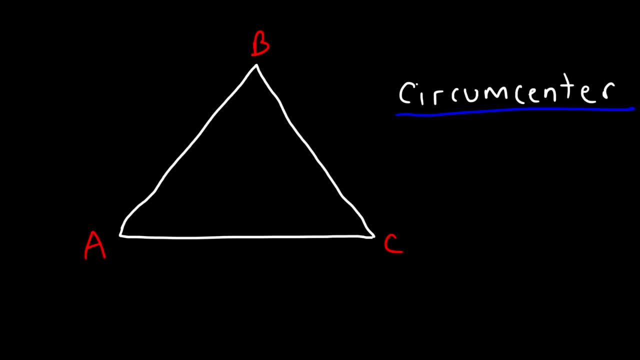 Let's call this triangle ABC. The circumcenter can be identified from the intersection of the three perpendicular bisectors of the three sides of a triangle, And it's very similar to the orthocenter In that It doesn't always have to lie on the inside of the triangle. 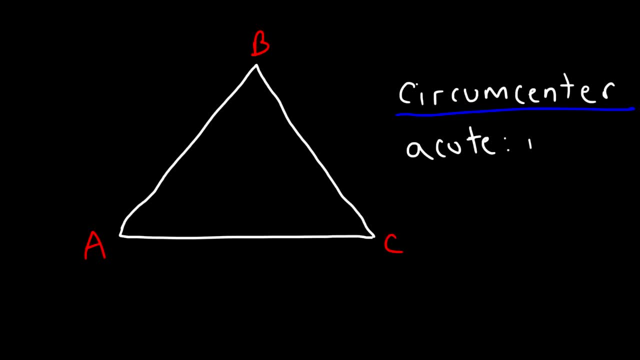 Now, if you have an acute triangle, The circumcenter is going to lie on the inside of the acute triangle. If you have a right triangle, It lies on the right triangle And if you have an obtuse triangle It will be located outside of the obtuse triangle. 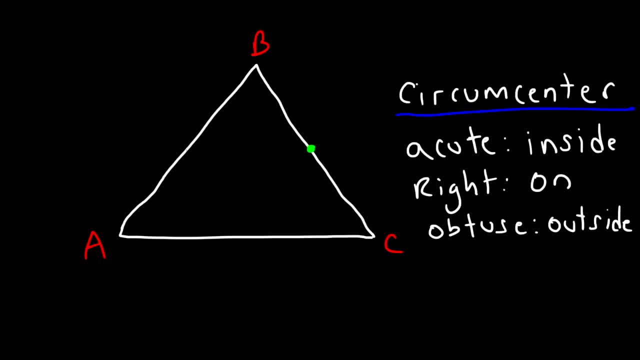 So first Let's identify the midpoint Of Each side. A perpendicular bisector is basically the combination of an altitude and a median. It has properties of both. So the perpendicular bisector for AC would be here. It doesn't have to touch a vertex B, Even though it may look like it's going to touch. 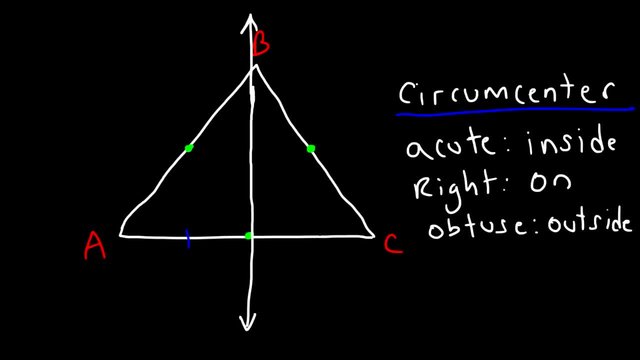 it. But, however, These two sides must be congruent, Because this point has to be the midpoint And also The two lines have to be perpendicular to each other. So let's draw something that's perpendicular to This side, OK. 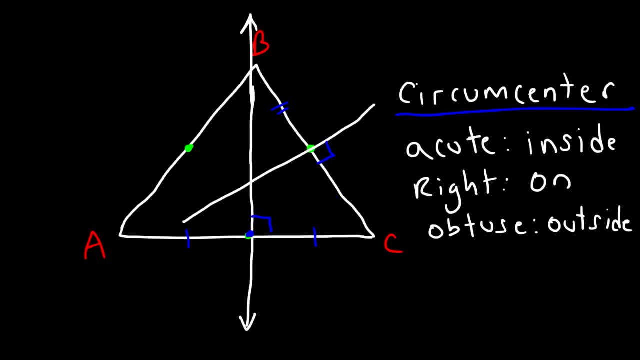 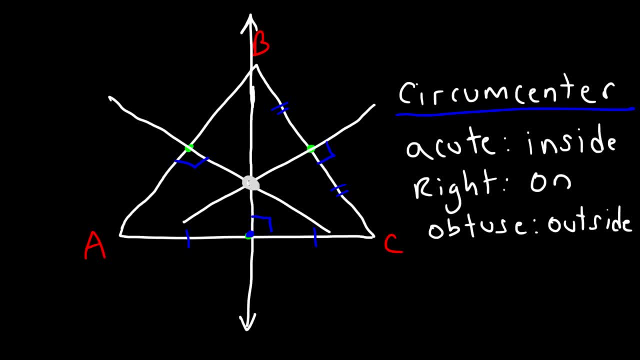 This, This, This, This, This, This, This, And this is approximately perpendicular to this side, So we can see that the circumcenter Is located on the inside Of an acute triangle. Now let's draw a circle, OK. 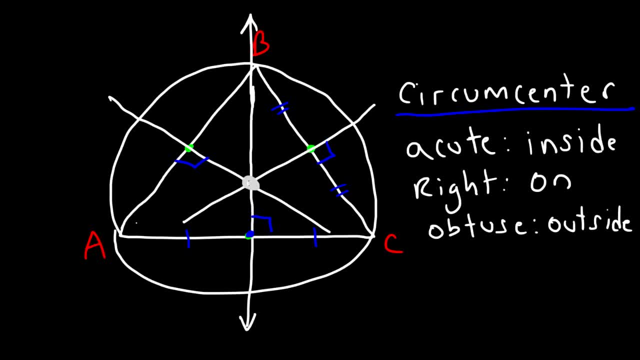 That circle wasn't looking good. So Notice that The that is circumscribed about the triangle. The in-center of a triangle is the center of a circle that is inscribed of a triangle. So hopefully you see the difference between a circumcenter and an in-center. 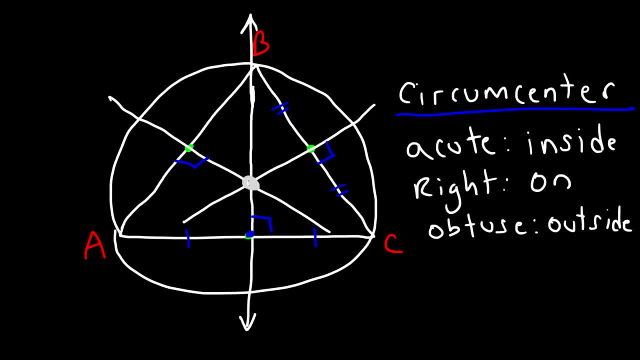 So, just to recap, the circumcenter of a triangle is the center of the circle when the circle is circumscribed about the triangle, And the in-center of a triangle is the center of the circle when the circle is inscribed, or inside of the triangle. 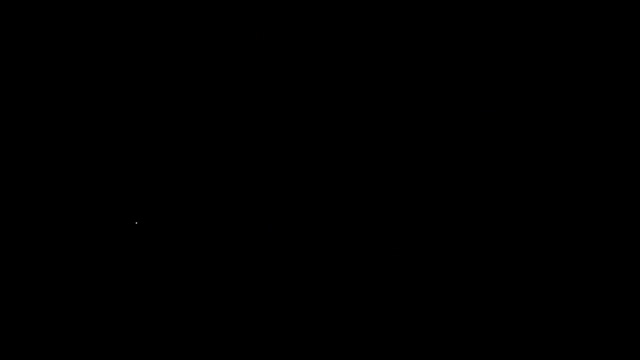 So hopefully that makes sense. Now let's move on to our next example, and that is the right triangle. So where is the circumcenter of the right triangle? So let's identify the three midpoints, Okay, And then draw a perpendicular line to each midpoint. 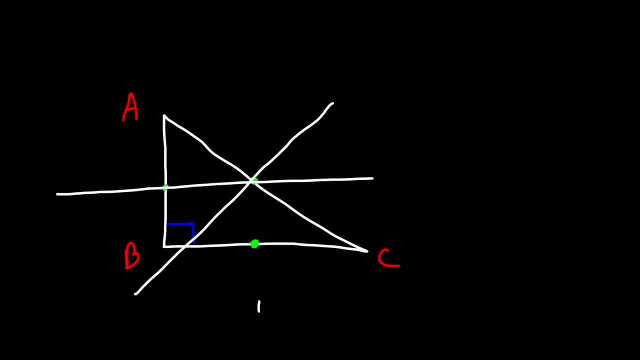 So we have a perpendicular bisector. So, as you can see, the circumcenter lies on the right triangle. In fact it's at the midpoint of the hypotenuse. So let's try this out. So this line is perpendicular to AB. 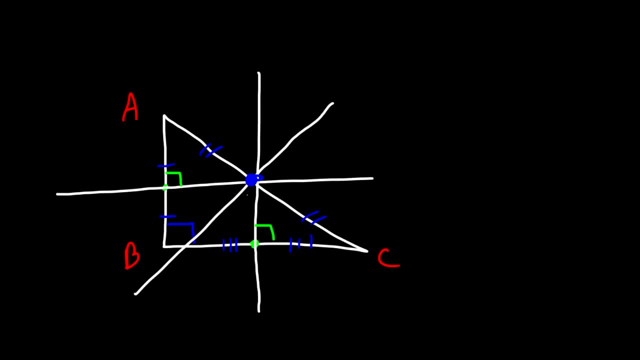 And this is the perpendicular bisector of BC, And here we have the perpendicular bisector of AC. So remember that The circumcenter can be found by the intersection of the three perpendicular bisectors. Now let's draw the circle. So it has to be perpendicular to AB. 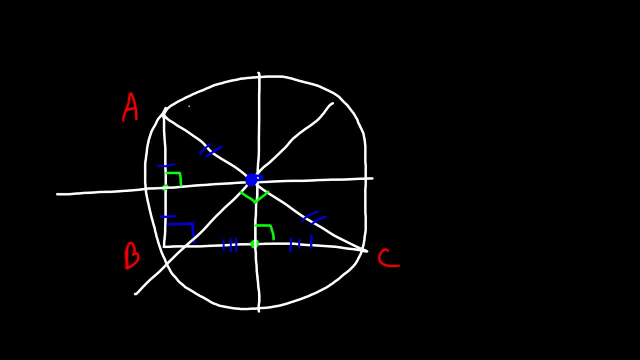 So here we have the perpendicular bisector to BC. So, as we can see, the circumcenter lies on the center of the circle that's circumscribed about the right triangle. Now let's move on to our next example, and that is the obtuse triangle. 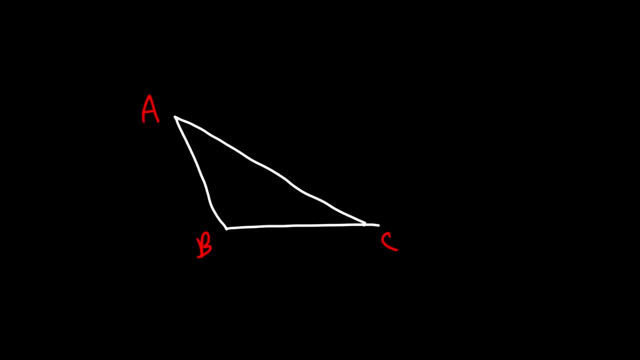 So this is A, B and C, And so first let's identify the midpoint of each side And then let's draw the perpendicular bisectors of those midpoints. Actually, that shouldn't be there, So we can see this is the right angle, this is the right angle and that's the right angle. 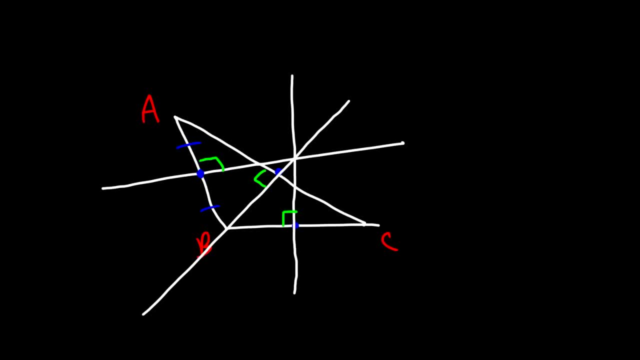 And then this point is the midpoint of A- B. These two sides are congruent, and those two sides are congruent. So notice that the circumcenter lies outside of the obtuse triangle. Now let's draw the circle. It should be something like that. 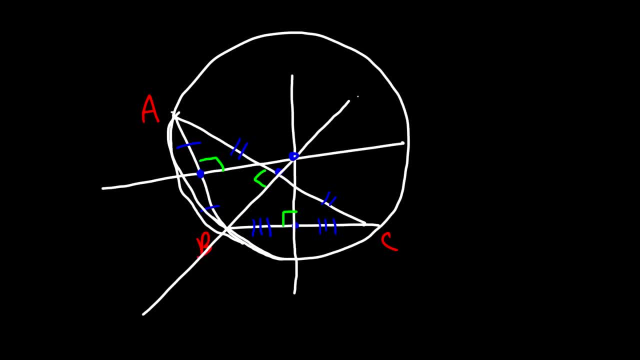 But, as you can see, my circle is not perfect, But if it was, you can see that this should be the center of the circle that's circumscribed about triangle A, B, C. So now let's review what we've learned so far.